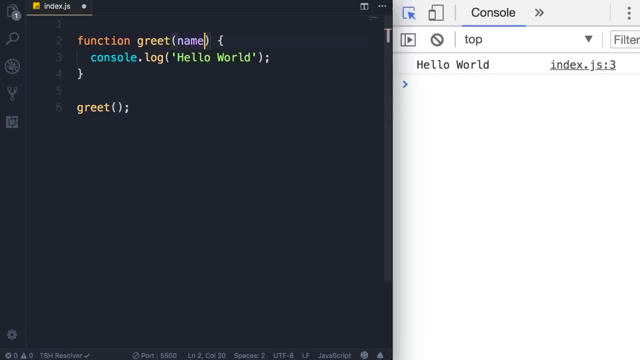 a variable. here, in between parentheses, we refer to this variable as a parameter. So this grid function has one parameter called name And essentially name is like a variable that is only meaningful inside of this function. So inside of this function we can. 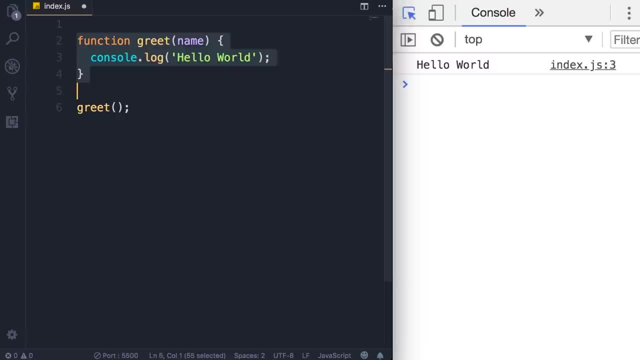 work with this name variable, but it will not be accessible outside of this function. Now, name is an input to this function, So instead of displaying Hello World, we can display hello. then add a plus here to concatenate two strings so we can add name after. 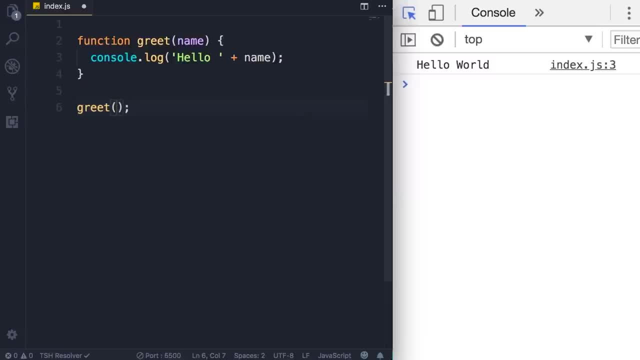 now, when calling the grid function, we need to pass a value for the name variable or name parameter more accurately, so we can pass john here. now we refer to this as an argument. so john is an argument to the grid function and name is a parameter of the grid function. that's one of 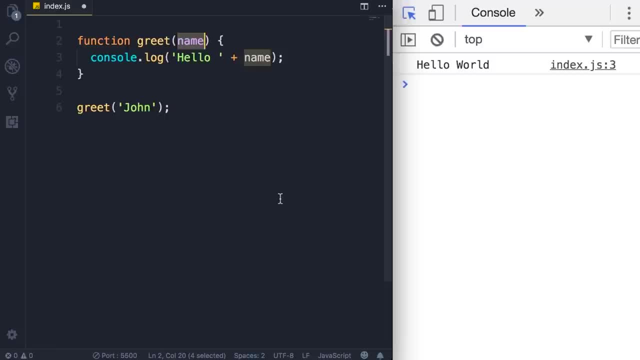 the things that a lot of programmers don't know. they don't know the difference between a parameter and an argument. so a parameter is what we have here at the time of declaration, but the argument is the actual value with supply for that parameter. okay, now let's save the changes. 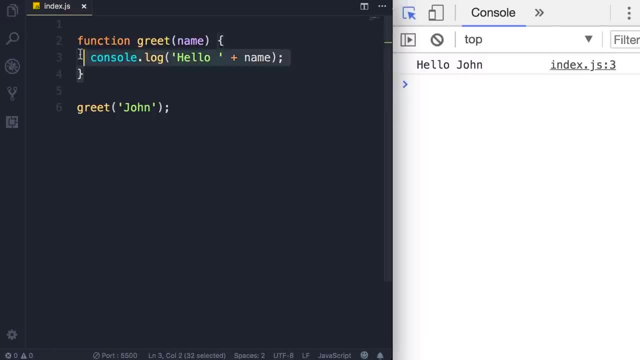 so we have hello john. now we can reuse this function, but with a different input. so we can copy this line here and change john to mary. save the changes. now we have two different messages on the console. now a function can have multiple parameters, so here we can separate parameters using a comma. so let's add another parameter like last name. 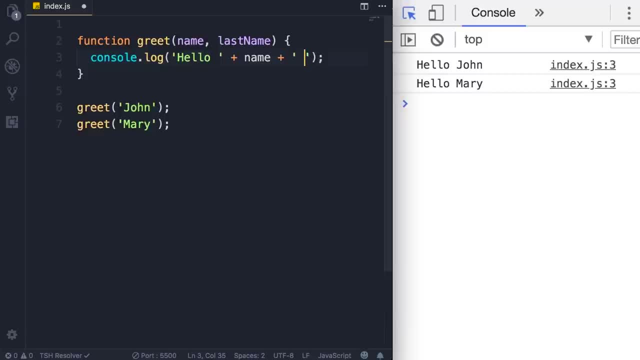 now we can change our consolelog, add a space here and then display the last name. now, when calling this grid function, we should pass another argument for the last name, right, but let's see what happens if we don't do this. so i'm going to save the changes. 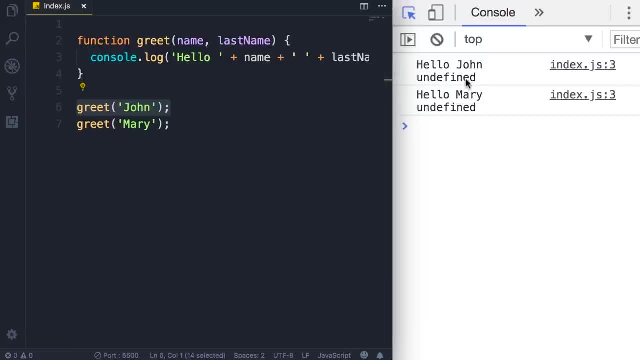 see what we got: hello, john. undefined. because, as i told you before, the default value of variables in javascript is undefined. so, because we did not pass a value for the last name, by default it's undefined. so i'm going to pass another argument here. we separate them using a comma, john smith, and we don't need the second call to the greet function.